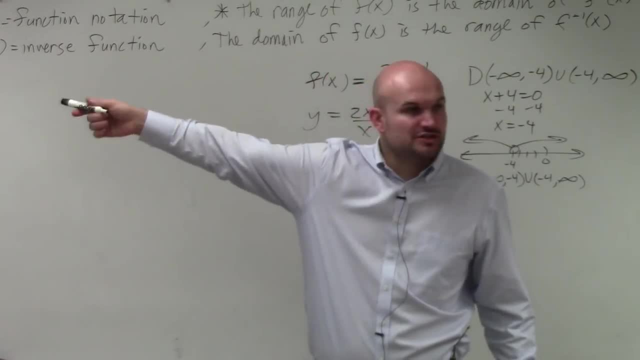 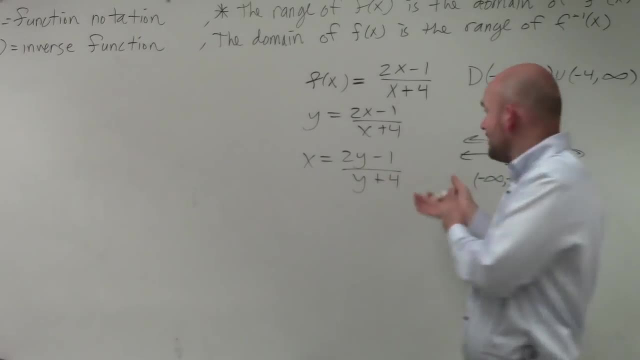 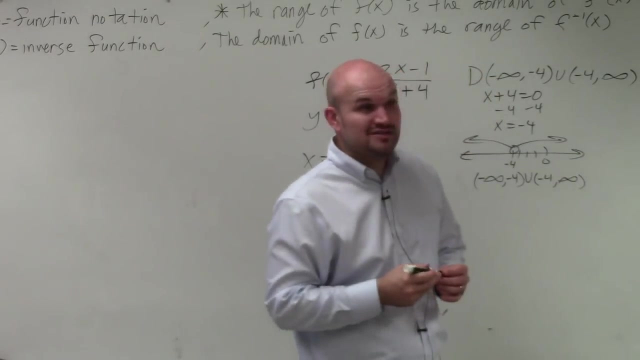 Remember, looking at the graphs, The x and y's are swapped from the function to the inverse. Do you guys agree with me now? Right, So that's graphically, you can see what happened Algebraically. that's how we're representing it is swapping our variables and now solving for y. All right, So going back to this equation over here that I solved from algebra one, If you have, you know, five over x, or if you have three equals five over x. you can't solve for x when it's in the denominator. So the first thing that I would teach in algebra one is you have to get the 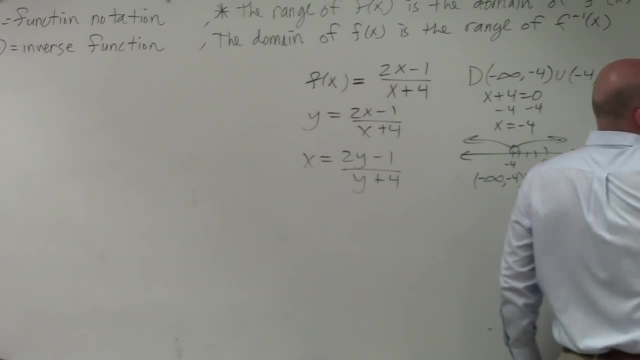 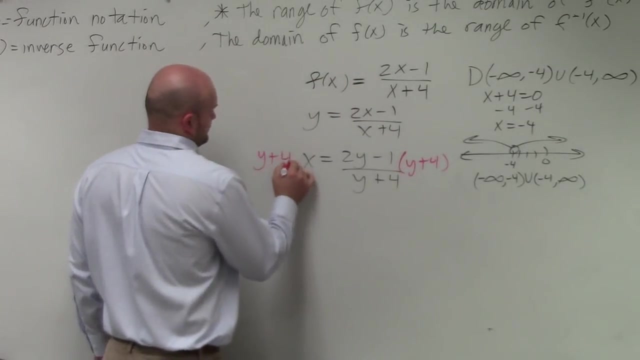 variable off the denominator. So multiply by x on both sides. When doing that, you get three x equals five. Now you can divide by three x equals five thirds. So I have y plus four in my denominator. I have to get y plus four off my denominator. So what I'm going to do is I'm going to multiply by y plus four on both sides. Since I have a y plus four in the numerator and a y plus four in the denominator, I'm going to multiply by y plus four on both sides. 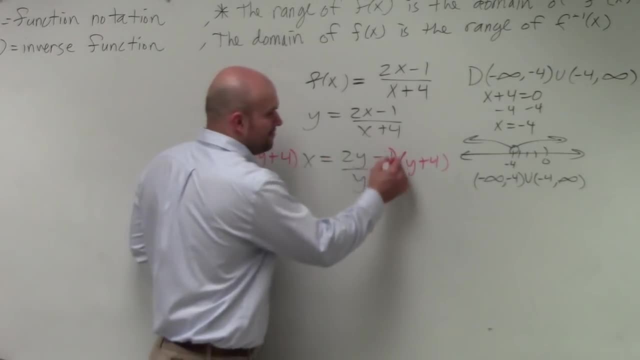 Since I have a y plus four in the denominator by the division property, I am multiplying these two. So that means these two are separated by multiplication. I can apply the division property and divide them. Did you have a question or a comment? 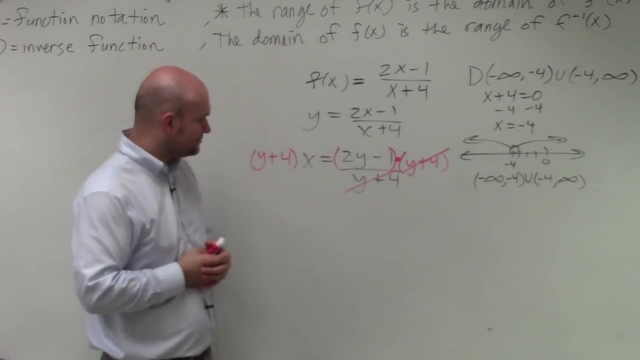 Okay, All right. Well, let me just finish and we'll kind of see how close you got. So now I can simplify this, but I also kind of want to get rid of these parentheses here. So I'm going to apply distributive property. So I get yx plus 4x equals 2y plus 4x. 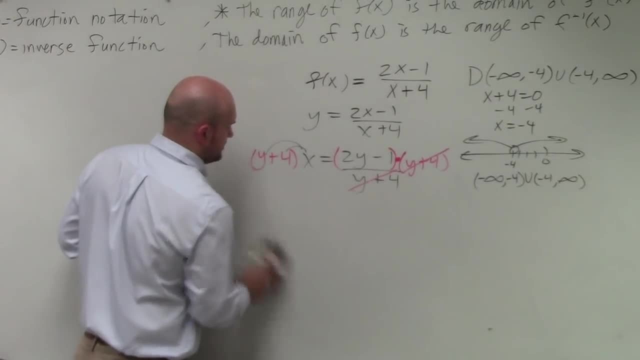 So I get y minus 1.. Let's do that a little bit lower down: yx plus 4x equals 2y minus 1.. Does everybody follow me in what I did so far? I think this is the point that you got to right. Okay, Now again going back to Algebra 1, if you have an equation, Yes, Kenny. 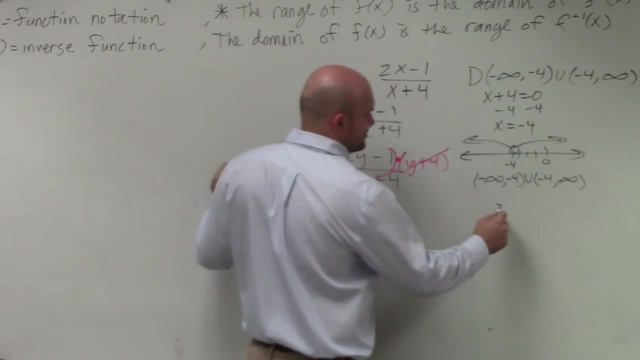 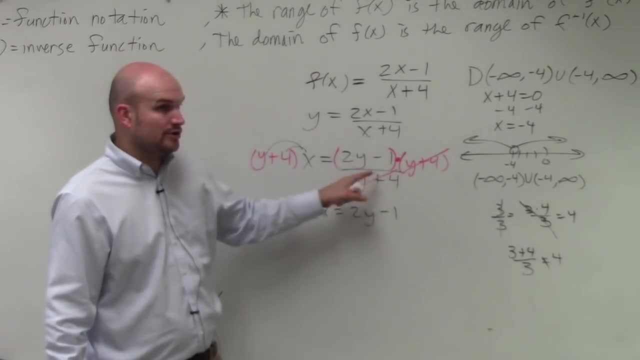 Well, yeah, I mean, what's 3 divided by 3 is 1. Right. 3 times 4 over 3 is 4. Right. Divide out, divide out. However, like 3 plus 4 divided by 3 is not equal to 4. Right, You can't cross them when they're separated by addition or subtraction. However, you might see addition and subtraction and say: well, you're doing that. No, I'm not. These two are separated by multiplication, So therefore I can apply the division property. 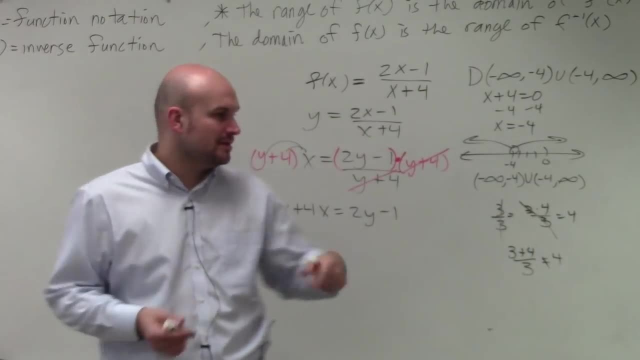 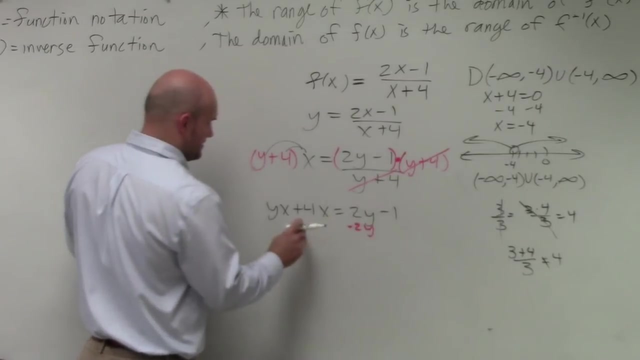 If you have a quantity divided by itself, it equals 1.. Now I need to solve for y, though I can only solve for y when they're on the same side, So I get them on the same side by subtracting. Now, in the problem I did, 3x and x were like terms, Right, I don't have like terms here, So I can't combine them. 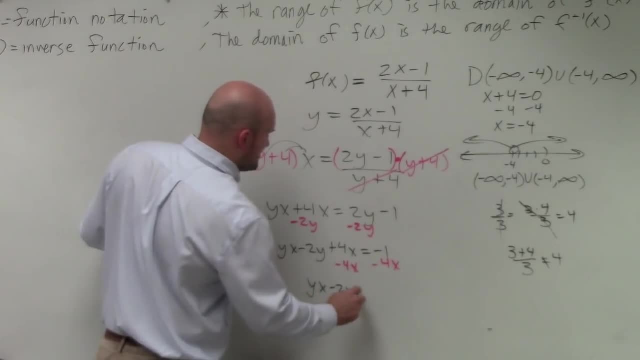 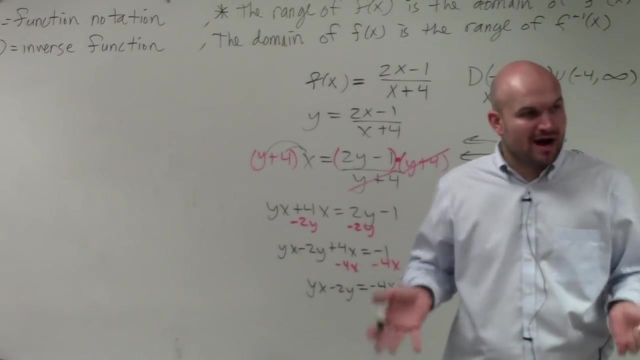 I could have done that at the same time, but I separated them, So I still have an issue, though, because I still have two y's Right, I need to get them down to one y. So what way can I solve for y? by getting this, Yes. 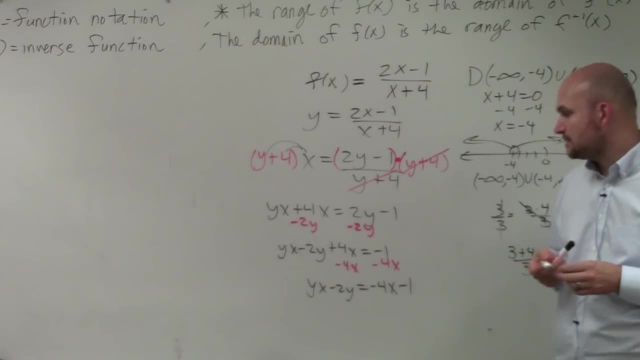 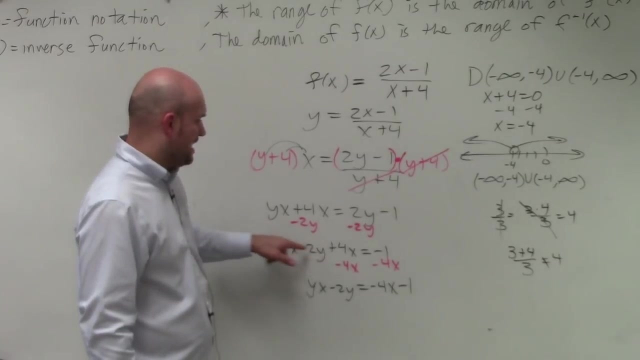 I knew the 4x over and I distributed xy out of x or I factored out yx out of yx, minus 2y plus 4x. Well, you can't factor, You can only factor a y out of here. But yes, but that's exactly the thinking that you need to do. Yes, 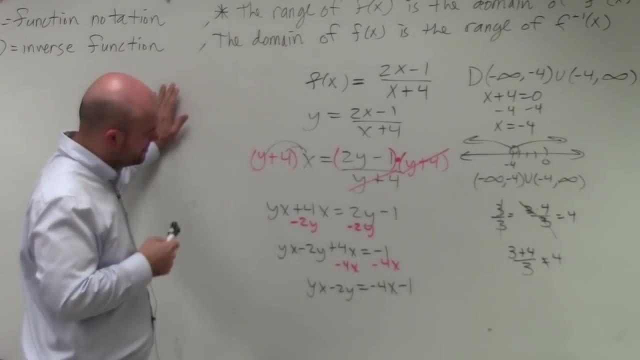 I moved all the terms that were with a variable to one side and then I factored out. My factorizing was x minus 2, for instance, and y plus 4.. Because I did kind of a complete square thing. I don't know what it's doing. It's really weird. 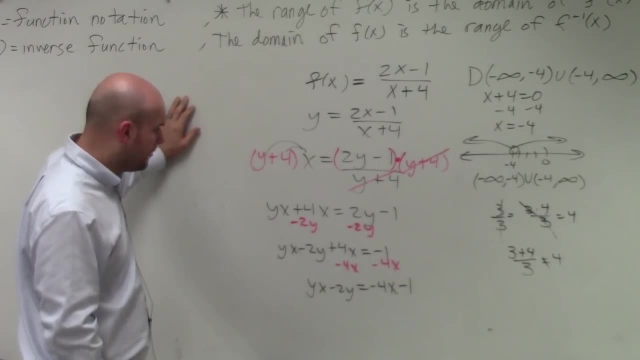 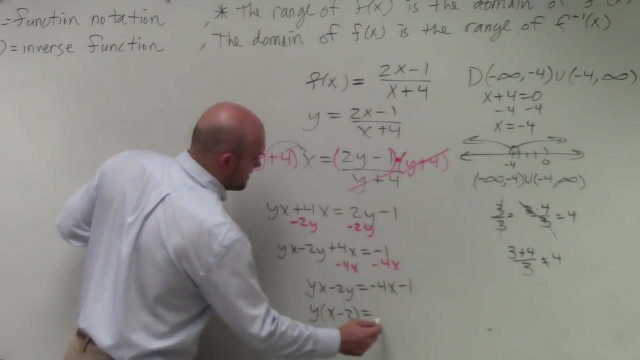 So you've got it factored or formed as y minus 2.. I'll have to go and check your factoring, but if you, I'll check your work here in a second. but if you just get the y's by themselves and then factor out a y, I'm not sure if you'll get the same answer as I did. or if you did, I'll have to take a look.